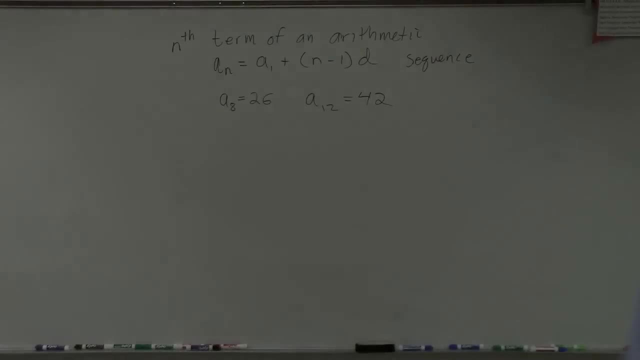 So we know that using this formula is going to become very, very important when we know that we have a consistent distance, which means it's going to be arithmetic sequence, all right. So for this problem, what they say is: they give us a of 8,, which is 26,, and they give us a of 12,, which is 42,. all right, 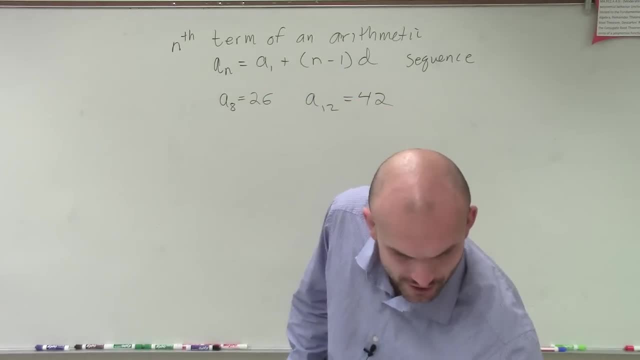 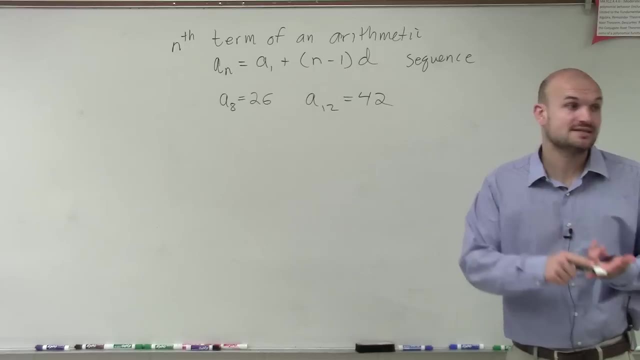 And what they're asking us to do for number 30,, for number 31,, they're saying, write the first five terms of the arithmetic series. So therefore, first of all, we don't know what a sub 1 is, we don't know what a sub 2 is, and we don't even know what the difference is right. 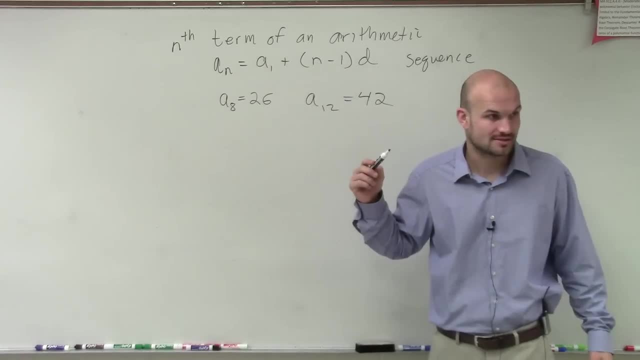 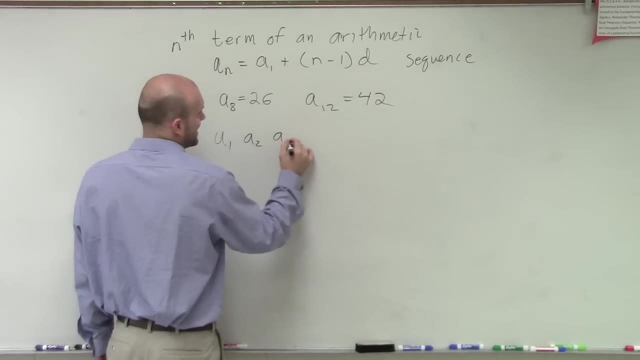 All we have is two numbers out of a whole sequence, correct? That's all we have Now. so let's go through this. If I had a sub 1, a sub 2, a sub 3, a sub 4, a sub 5.. 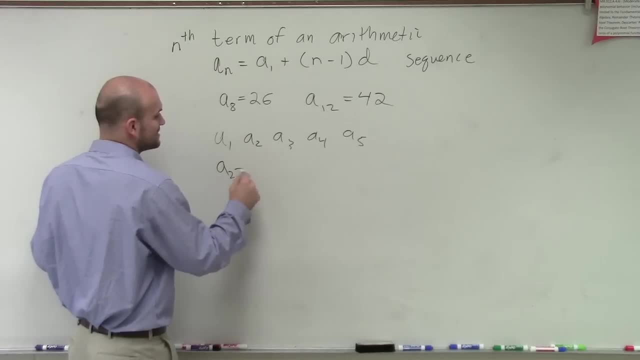 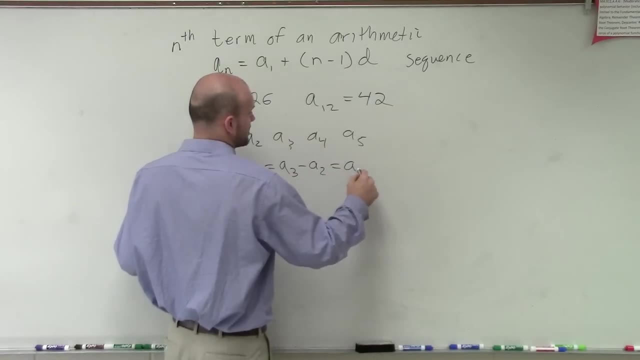 Remember, we know this is an arithmetic sequence. So therefore we know that the difference of a sub 1 minus a sub 2 minus a sub 1 is equal to a sub 3 minus a sub 2, which is equal to a sub 4 minus a sub 3, and so on, and so on, and so on, right, 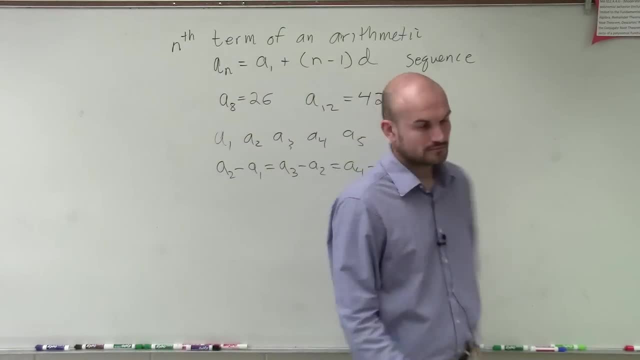 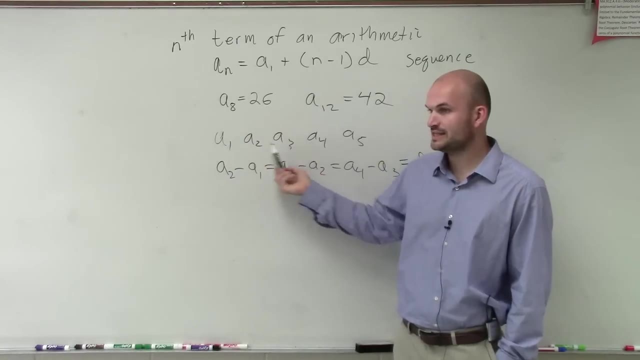 All those values equal d. Now here comes my issue. If let's say the difference between these two is d, the difference between these two is d, these two are d and these two are d, right, Yes? So, ladies and gentlemen, then you're going to have to do this. 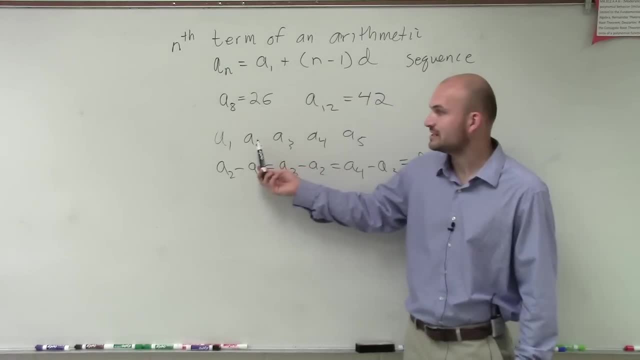 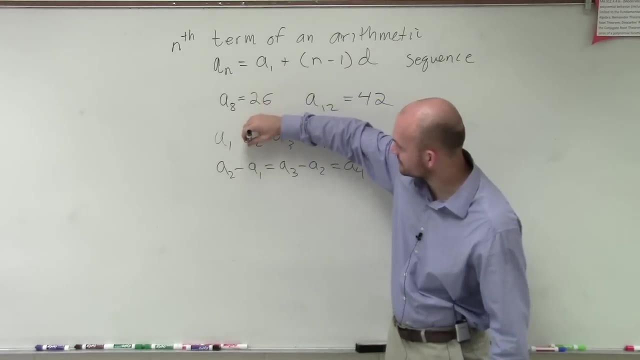 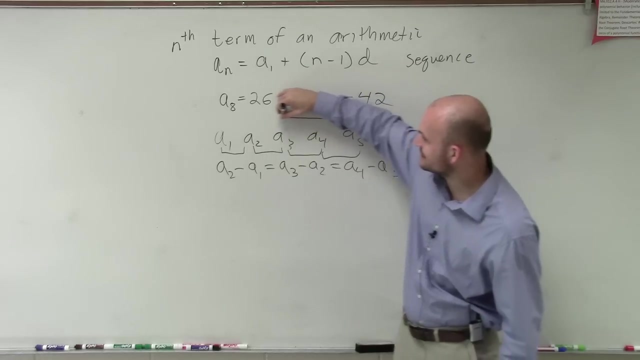 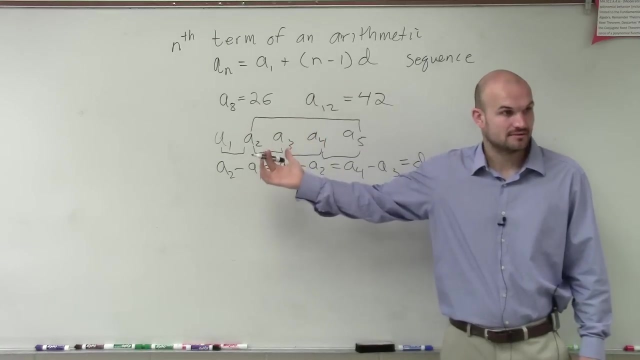 So, ladies and gentlemen, then you're going to have to do this, And does it make sense, Let's say I'm only given the difference between, let's say, I'm just given two values. Does it make sense, though, if I can find so, if I know the distance between all these is d? does it make sense then, if I find the distance between those two terms, that I can find the difference between those two terms and then divide it by 3, and that will give me d right? 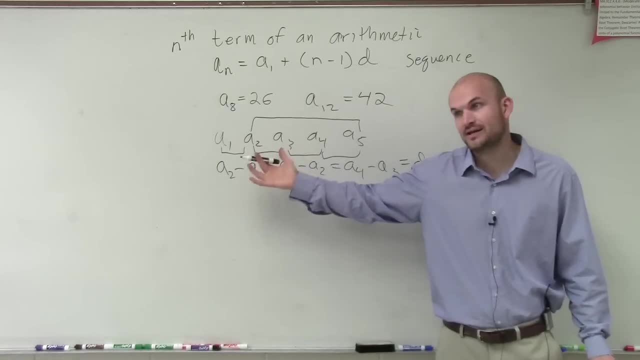 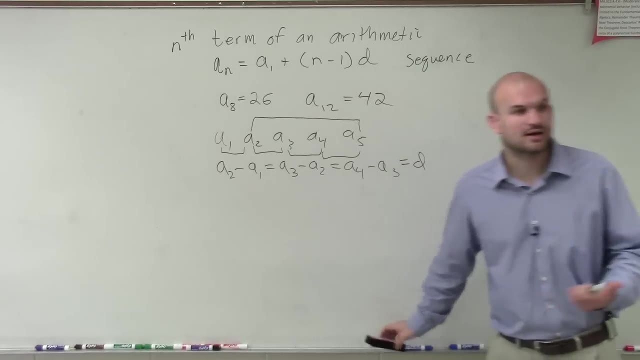 Does that kind of make sense? I can find that difference, I can find that distance and then divide it by how many distances I have, and that would be. you know, that would give me d okay. So that's exactly kind of what I'm going to apply here. 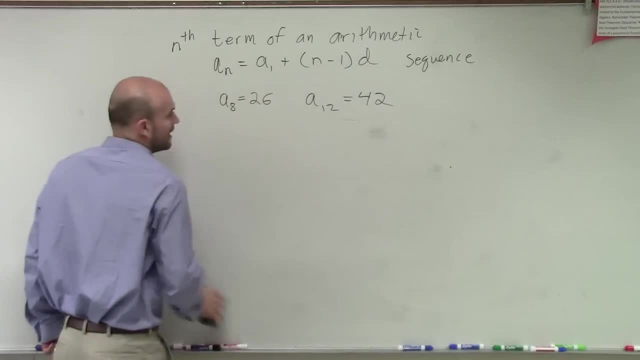 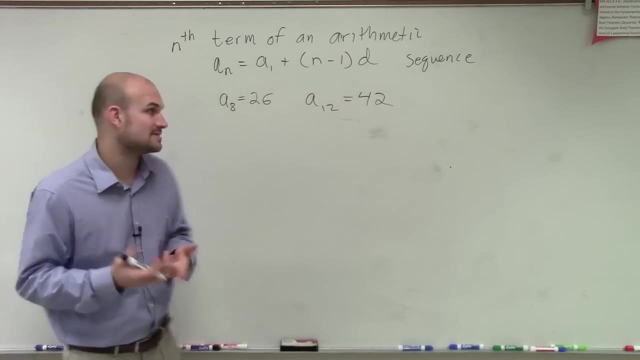 Zach, what I'm going to look at is: I'm not given, I don't know what d is and I don't know what a sub 1 is, but I have to be able to figure out what the difference is. I have to be able to figure out for me to find out what a sub 1 is. I have to know where am I going.